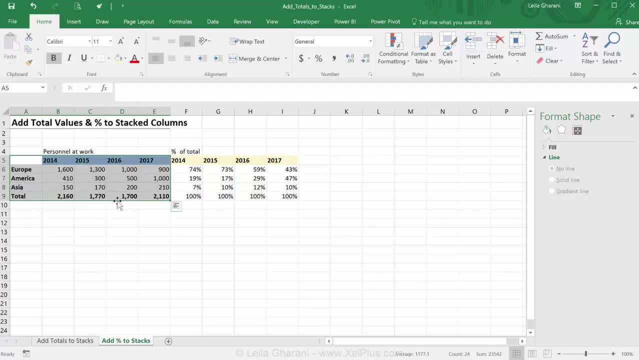 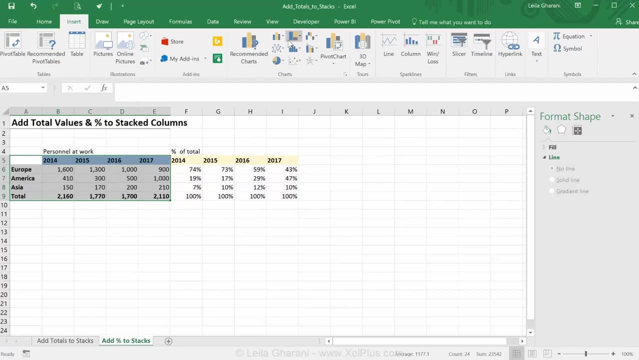 and then I calculated this and I brought it in. But once you know how the techniques work, you can just do it all in one step. So just highlight everything. insert a stack column. Okay, that's our total stack, so it's added it as a last stack column. 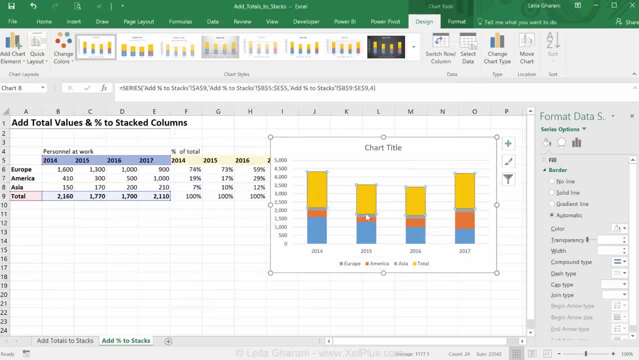 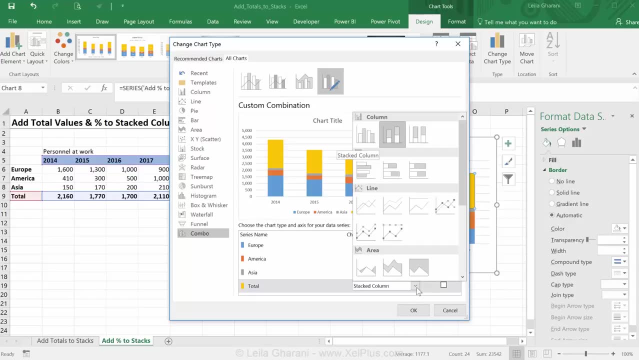 on top of everything else, all we have to do is to change the series chart type Of this total series instead of a stack column. I took in the last video. I took a scatterplot, but I'm going to show you that it works just as well. 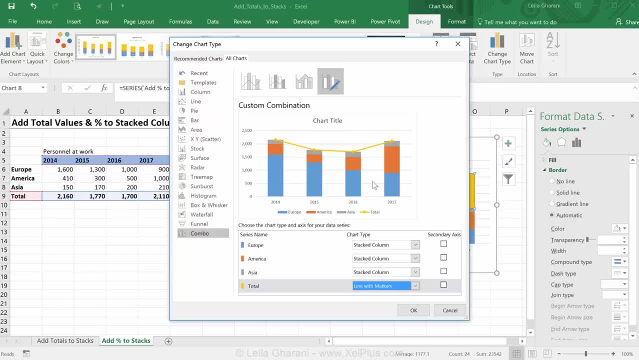 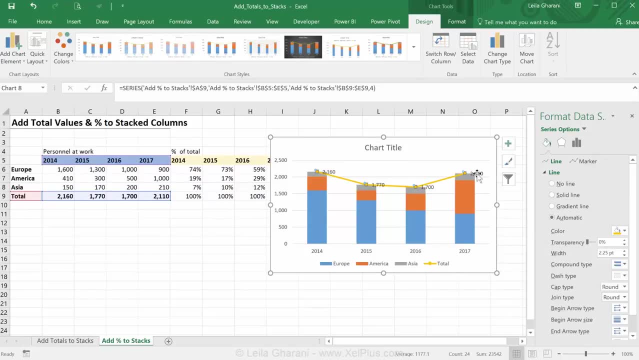 with a line chart, so I'll just pick this one line with markers. Now for this series, I'm going to add the data labels and let's position them so they're on top. Let's just go and make them bold and bigger. 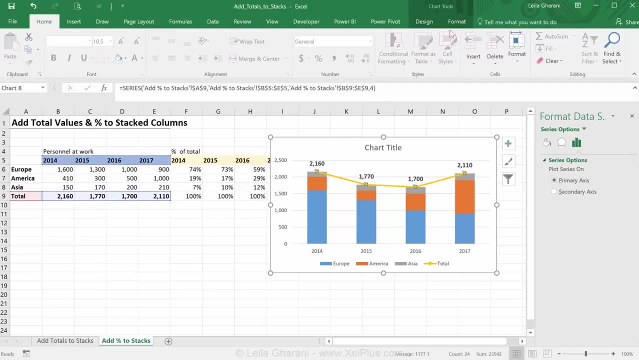 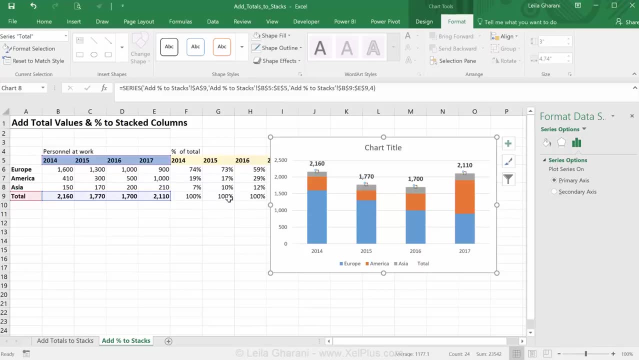 and I'm going to hide this series here. I can just go to format and shape outline. I think that's already there. so no outline and shape fill. no shape fill. That takes away the markers and the lines. So let me just remove these. 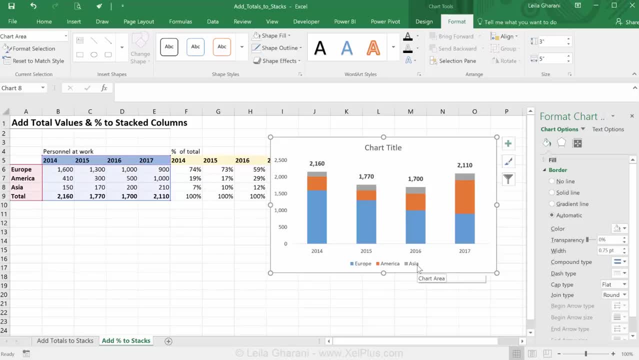 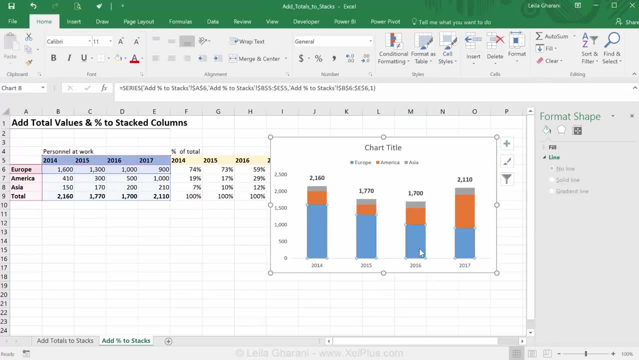 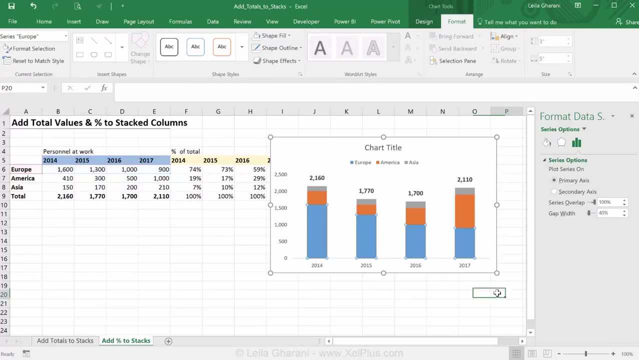 And this total. I don't need it, so you just click, click and delete. Now I'm going to push this to the top. Okay, that looks better. Let's just decrease the gap width here. I'm just going to go a bit dramatic and go to 40%. 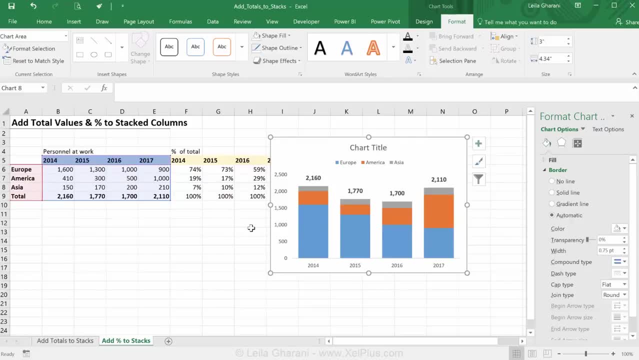 Okay, you can make the whole chart a bit smaller. Okay, so now I'm going to add the data labels to these, but I want these as well. Now, it really depends on the version of Excel that you have and the technique that you like. 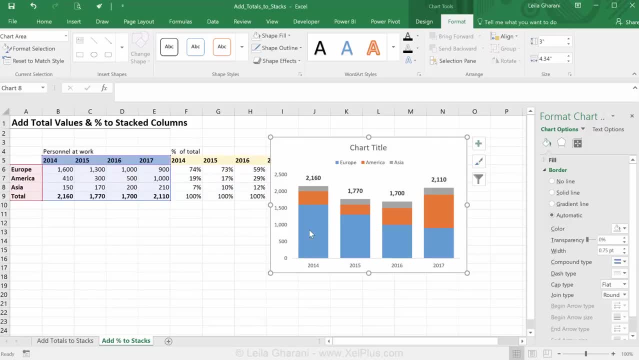 So I'll just show you different ways of adding this. One technique that works for Excel 2013 and above is first of all, add the data labels. then, when you go to format the data labels, go to options, label options and select value for. 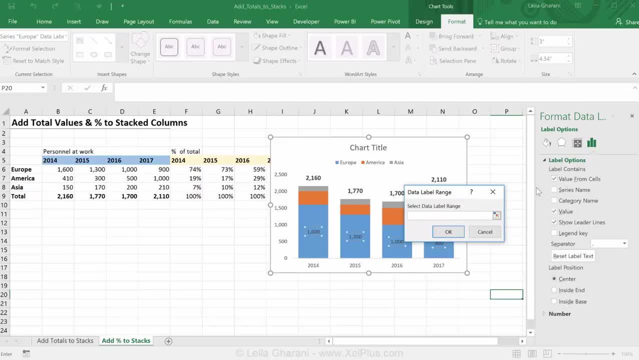 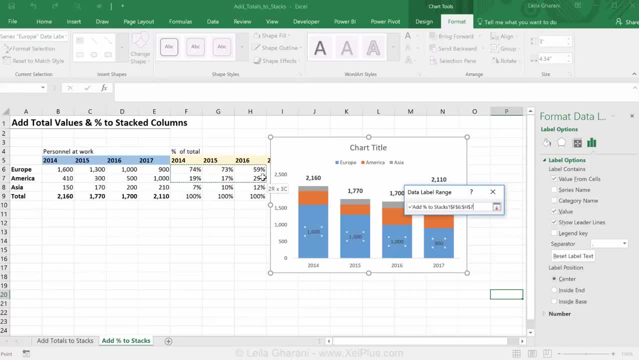 Go to options, label options and select value, for, In this case, this is Europe. I'm going to select this row here and say, okay, Now I'm going to leave the tick mark on value, because that's the original value here. 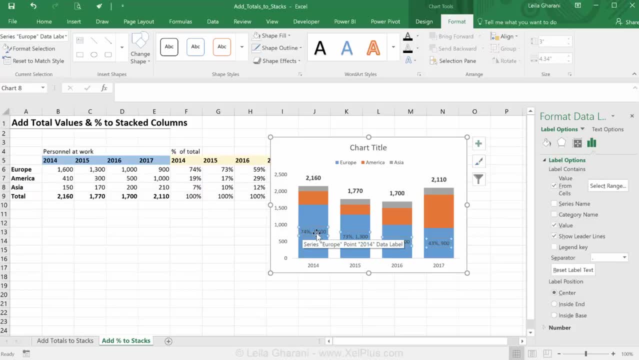 Now I'm showing percentages and I'm showing the value. It might be too cramped in this way. I mean, right now with my thicker bars it looks fine. but what you could do is define your separator to be a new line and that way you push it down. 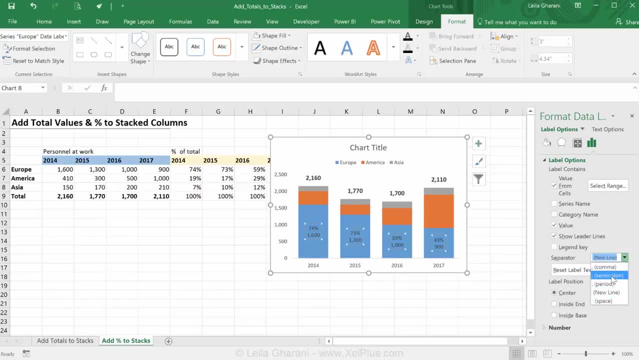 You see you have some separator options here. by default it's a comma, but you can pick period, semicolon or space. I picked a new line here. This works for Excel 2013 and above. Now let's say that you have an older version of Excel, or you also want to add your own type of separator, or 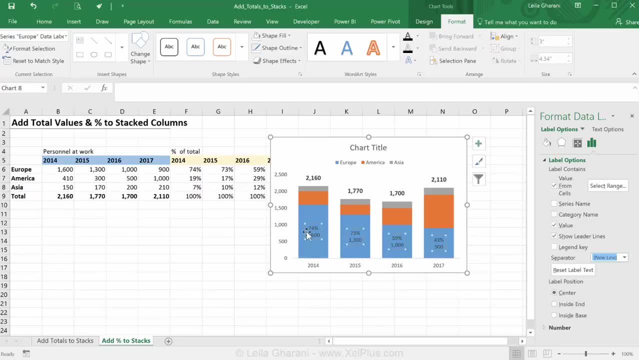 you just want to add your own type of formatting. So let's say you just wanted the percentage part to be in brackets. You can't find that type of formatting here. What you could do is to add your own labels. I'm just going to copy these. 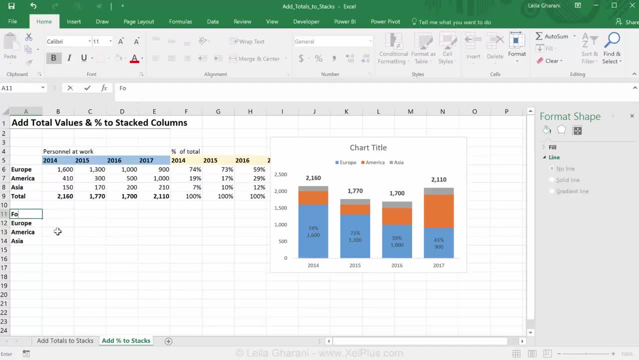 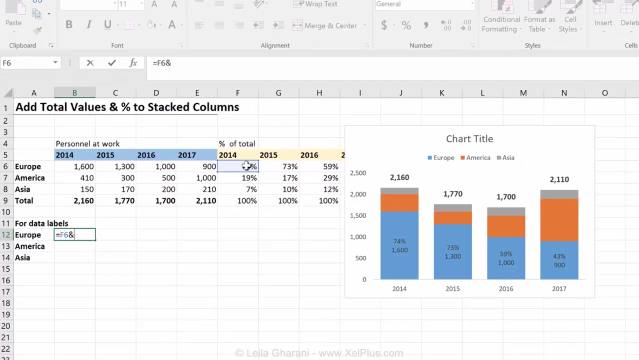 paste them here and say: for data labels, I'm going to add my own labels here. What I want is to have this number and have a space first and this number, and I want to put this number in brackets. Basically, I'm going to start and say: 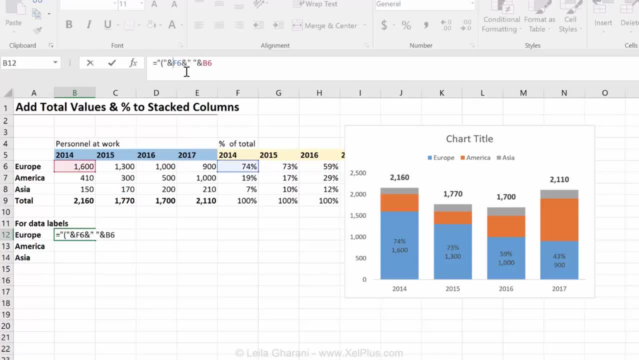 equals bracket- open quotation mark and then my number, and it's a lot of ands there, but that's how you combine text with cells. You always need these quotation marks. So I'm going to say bracket, closed quotation marks, and that one. that should be fine. 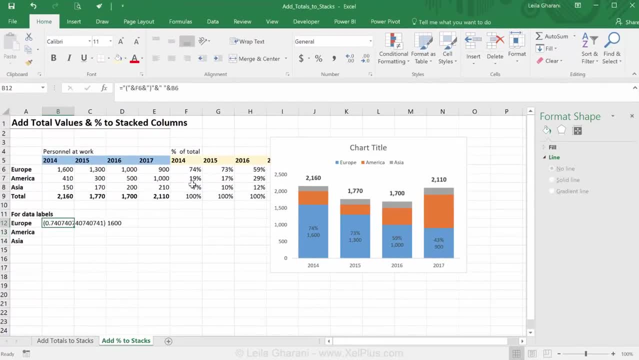 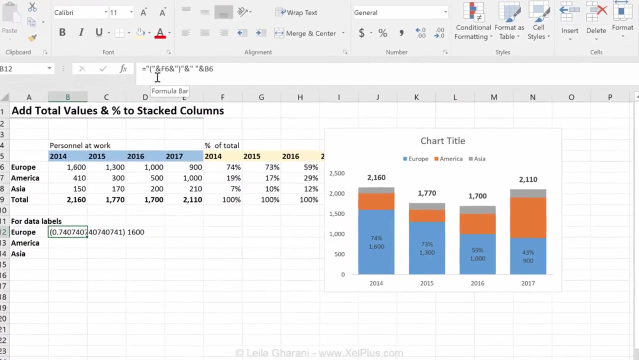 Okay, so it's putting my brackets, but it's showing the full number here, because the formatting of the cell when you're combining different numbers, it reverse to general and I have different numbers and I want to format them differently. So the function that works great here is the text function. What I can do is to wrap this one in. 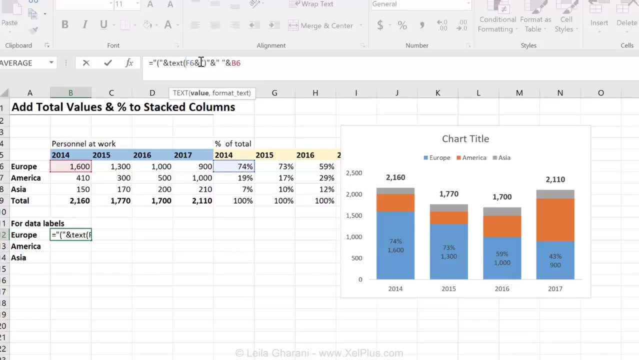 a text function that says: format this one cell as a percentage. That means I need to define zero. Zero is just a placeholder for the number and percentage. I don't want any decimal places. Okay, so that looks okay. Let's just check. 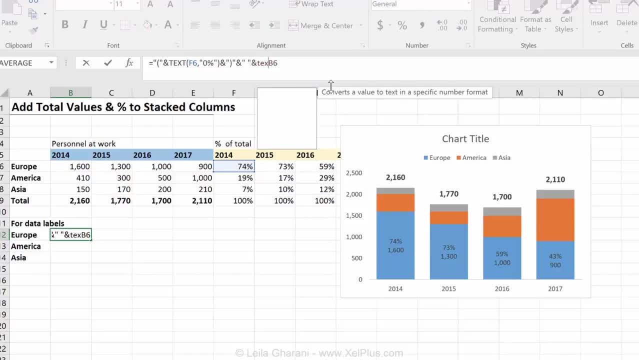 Okay, that works. Now for the last one. I'm going to do the same thing, but I don't want to show it as a percentage. I want to show it with a thousand separators, So I'm going to use the hashtag sign for a placeholder as my number, and 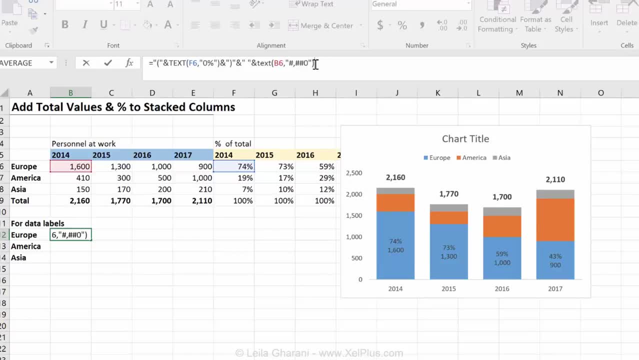 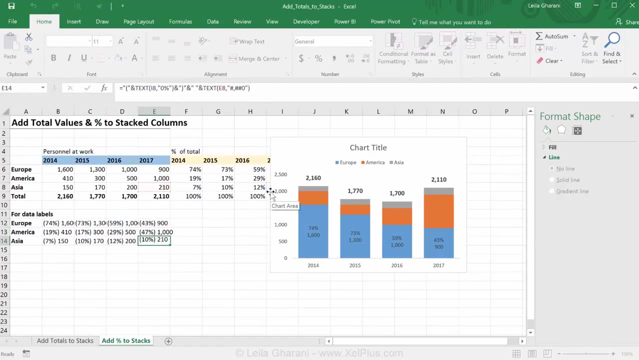 the zero for the last one, and that should work. I don't need to fix any cells, I can just drag this along and drag it down. Okay, let's just double check that the references are okay, and that's the one right behind my chart. 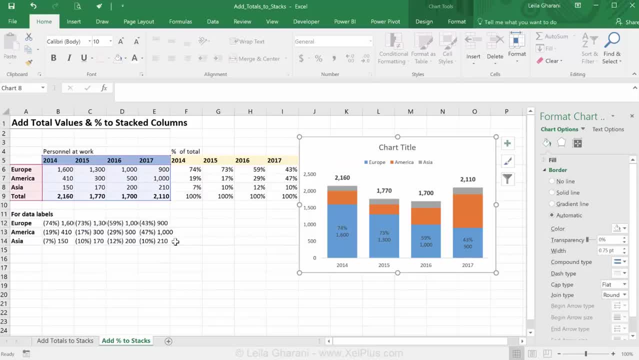 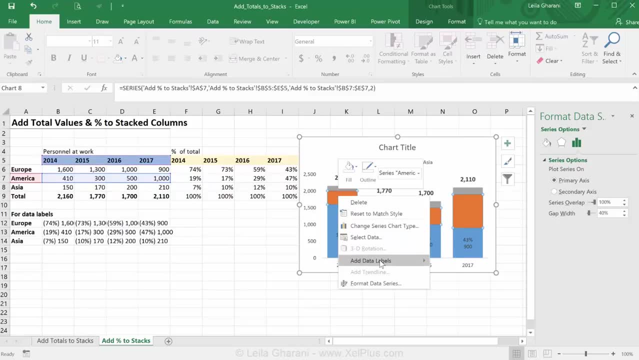 Okay, let's just make sure it's 10%. that looks good. I have my own type of formatting. let's bring it in. I'm going to right mouse click, add data labels. so you always need that before and then you can format the data labels. 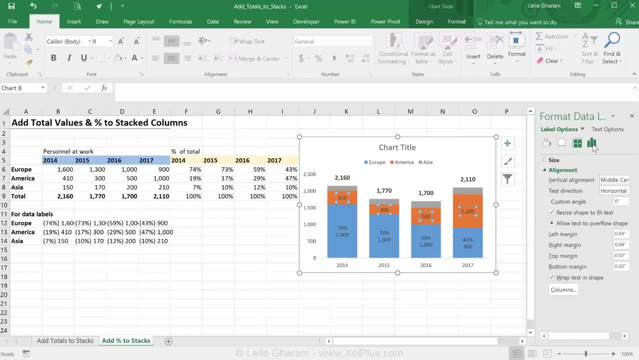 to show what you want. This technique that I'm going to show you right now is again for Excel 2013 and above, but I'm going to show it to you for this last stack. I'm going to show you how it works with Excel 2010. 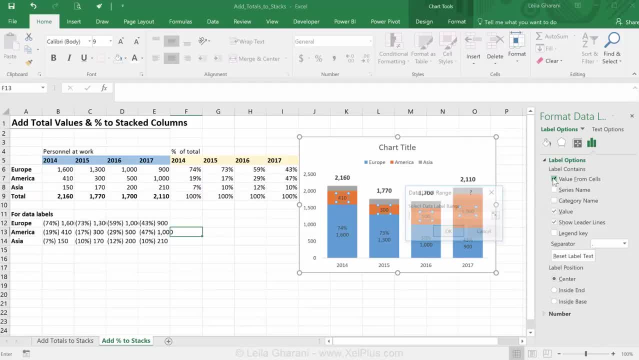 or Excel 2007.. Here we're going to say value from cells and we're going to select. now I'm in the second one, America. we're going to select this one and okay, Okay, but this time I don't need the value. 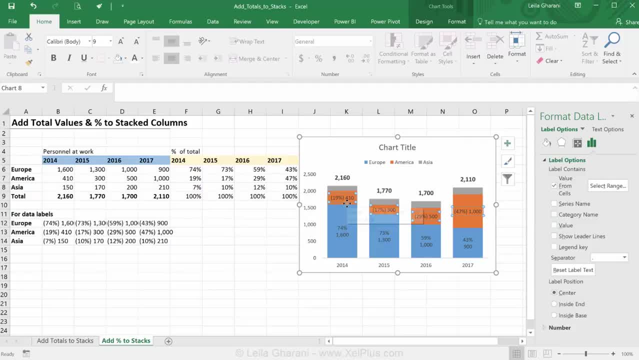 so I can uncheck this. Leader lines I don't need either, can't see them anyhow on this. but how do I get a line break in here? now I can try with this separator and say show new line, but it's not showing. 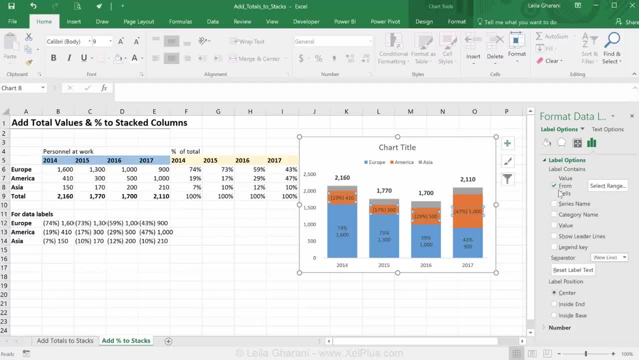 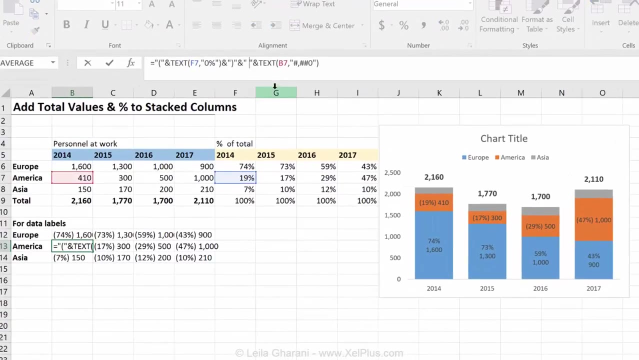 more than one thing. that separator works if you're showing more than one category, one name here, and I'm not. I'm showing everything in one. I actually want to generate a line break in here, and I can do that using the Alt and Enter key. 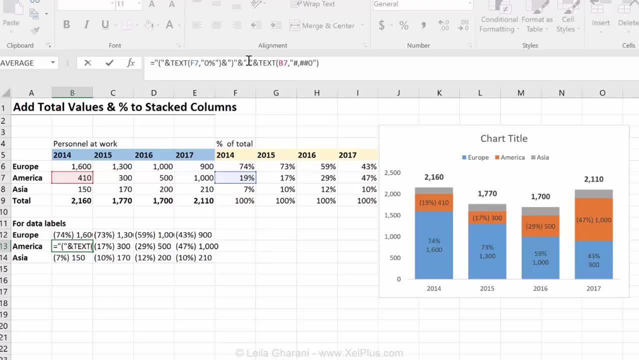 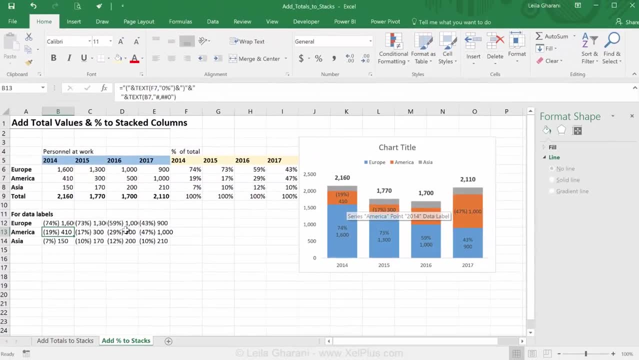 so right here in this text, where I have my space, I'm going to click and I'm going to press Alt Enter and then press Enter and that generates that line break and I can copy it across. Okay, so that still works in this stack. 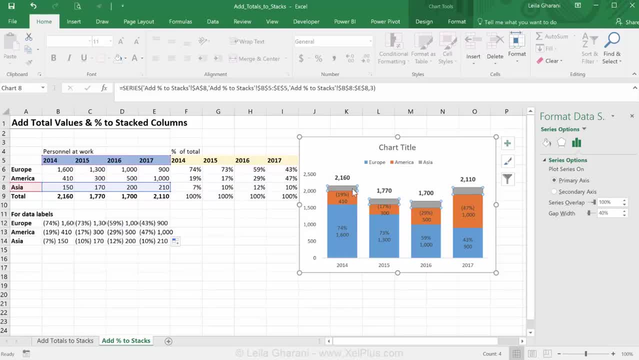 Now, in the last stack, I'm going to show you the method for Excel 2007 and 10.. Again, add the data labels to it. then click on the data labels. but now what you need to do, because you don't have this option available. 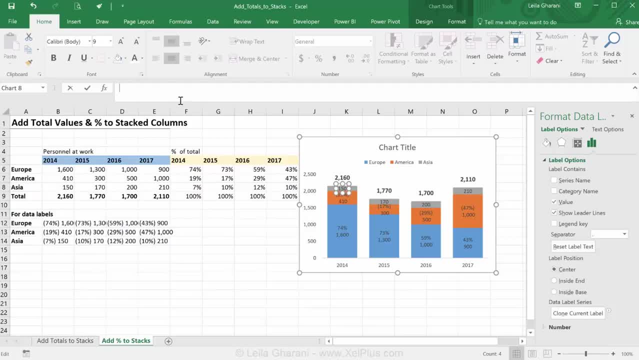 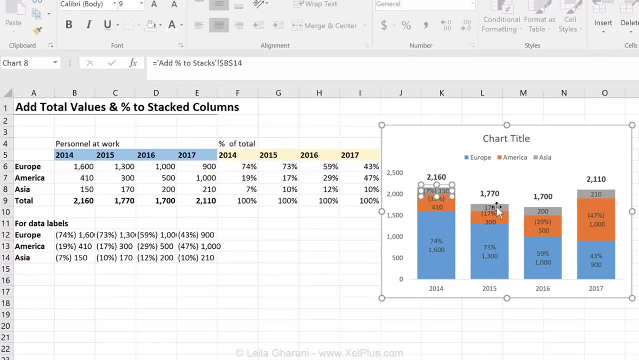 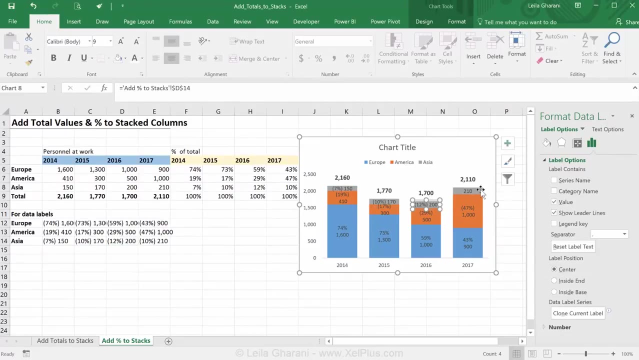 what you have to do is this: you have to click again on the first label, go to the formula tab, press equal and select your number- so that's my 2014,- and then do the same for the next ones, In this case, because this is a smaller stack anyhow. 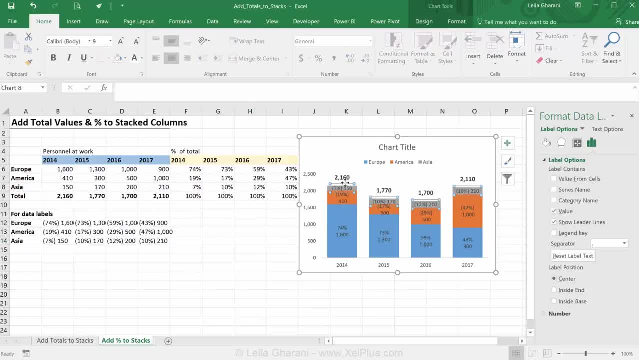 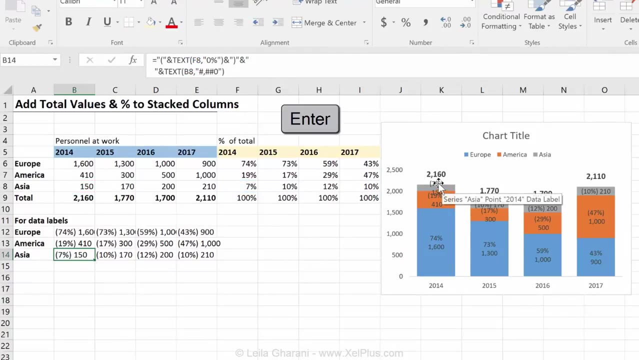 I don't need to generate a line break, but the line break technique works also when you use this technique. If I wanted to generate a line break here, I can just go into Excel and I can do that my same. go to this data label, press Alt and enter and enter, and then it reflects it here. 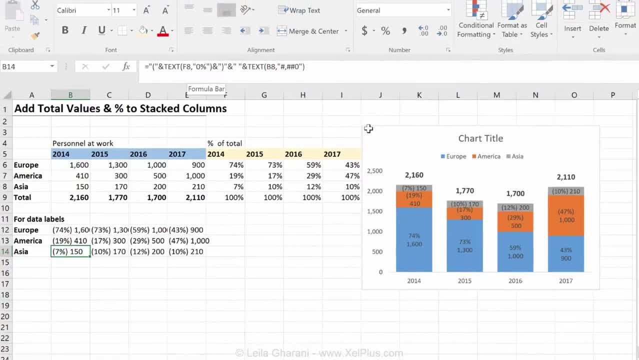 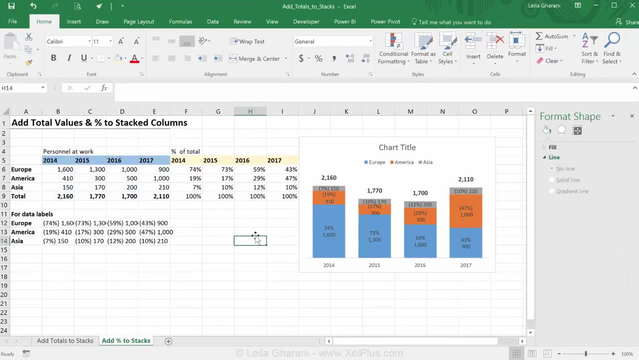 Okay, but in this case I don't want to do that. Now that I'm showing both, I can actually remove the y-axis. These are different ways that you can show more than one data label in each of your stacks. The version that you choose really depends on what you prefer. 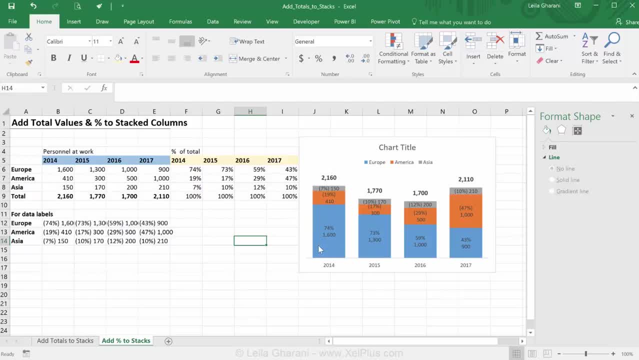 and also on the version of Excel that you have. For me this is a little bit too crowded. It's just too much data in the chart. I prefer to restrict it to one data label and then show the other part, the other values that I want to show in a different way. 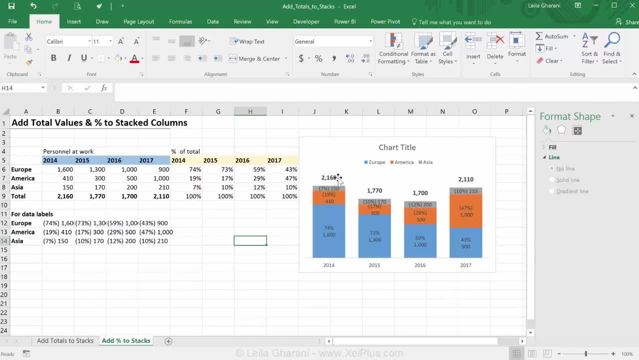 Here. let's say, the important thing to show is the total values here and the percentage contribution of each of the stacks. The way I would prefer to show this is like this: I'm just going to copy this chart and paste it down here.